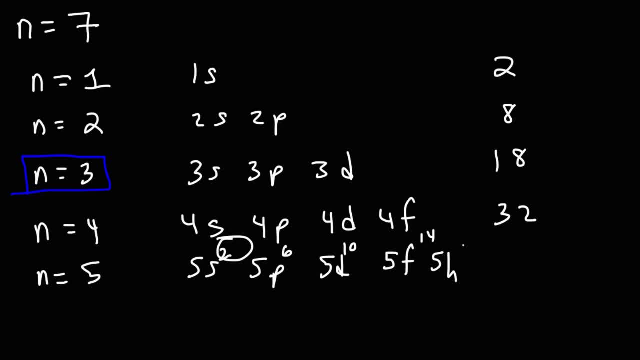 increasing by 4.. 14 plus 4 is 18.. So h can hold up to 18.. If we add 32 to 18,, we get 50. Now what is the relationship between these numbers and their respective n values? 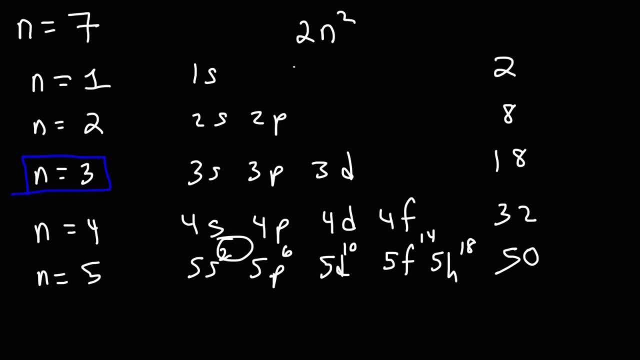 Notice that it's always 2n squared. For instance, when n is 3, if you square it, you get 9.. 9 times 2 is 18.. When n is 5,, 5 squared is 25 times 2, you get 50. So when n is 7, the maximum number of electrons 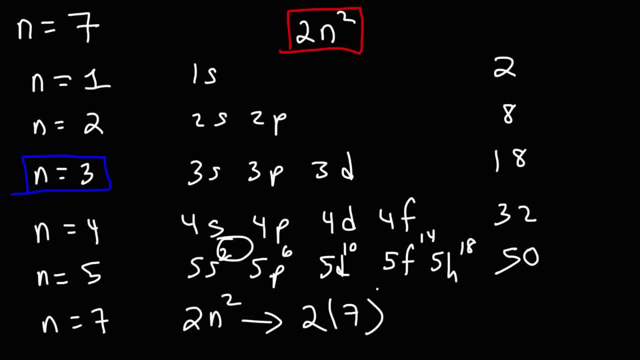 is going to be 2n squared, or 2 times 7 squared. 7 squared is 49.. 49 times 2 is 98.. So the maximum number of electrons in the 7th energy level is 98 electrons. 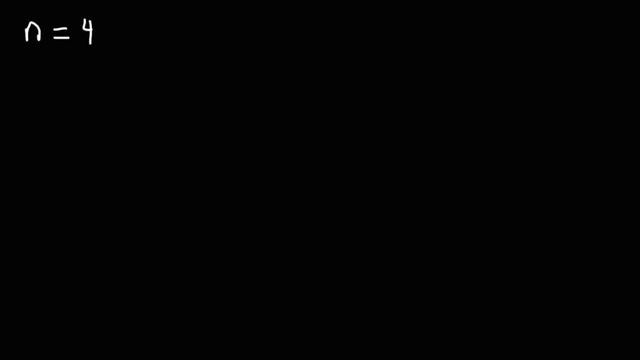 Now let's move on to our next example. So let's say that n is 4, and ms, that is, the electron spin, is positive 1 half. What is the maximum number of electrons with these two quantum numbers? How many electrons? 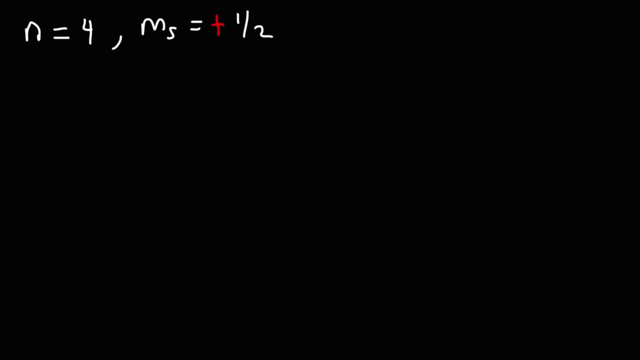 How many electrons can have those two quantum numbers? Well, we know how to determine the maximum number of electrons in the 4th energy level. The answer is going to be 2n squared, So it's going to be 2 times 4 squared. 4 squared is 16. 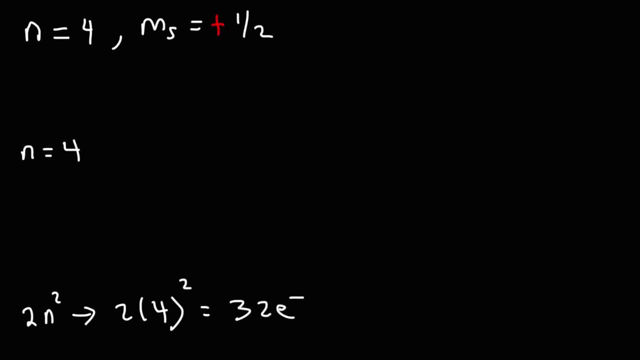 times 2.. So there's a maximum of 32 electrons in the 4th energy level. Half of them will have a spin of plus a half, That is, half of them will have an up arrow. The other half will have a spin of plus a half, That is, half of them will have an up arrow. 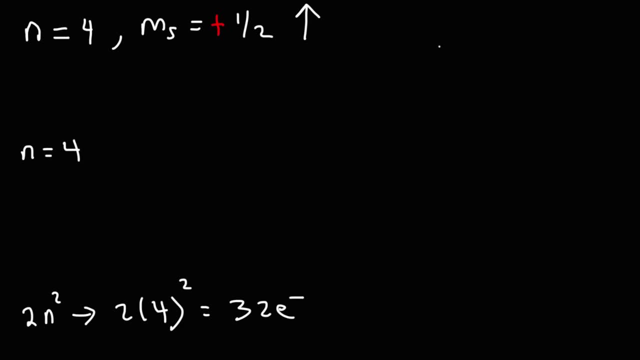 The other half will have a down arrow. So the answer is going to be half of 32 electrons. It's going to be 16 electrons. Now, for those of you who want to see the answer visually, here's what you can do. So the 4th energy level has four sublevels. It has the s sublevel. It has the p sublevel. By the way, the p sublevel has three orbitals. It has the d sublevel, which has five orbitals, And also the f sublevel, which has seven orbitals. Each orbital can hold a maximum of two electrons. 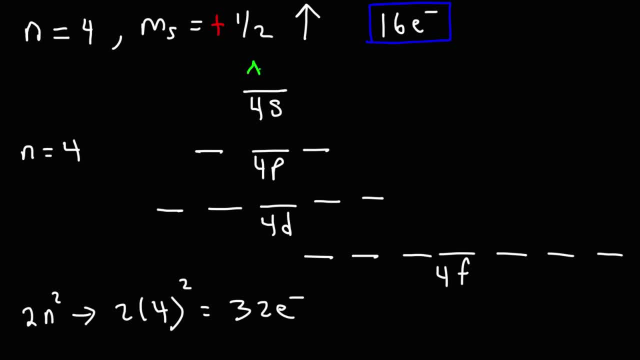 So in each orbital there's going to be an up arrow and a down arrow. So if you were to count all of the arrows in the 4th energy level, you should get a total of 32.. So you have 2 in the s sublevel, 6 in the p sublevel, 10 in the d. 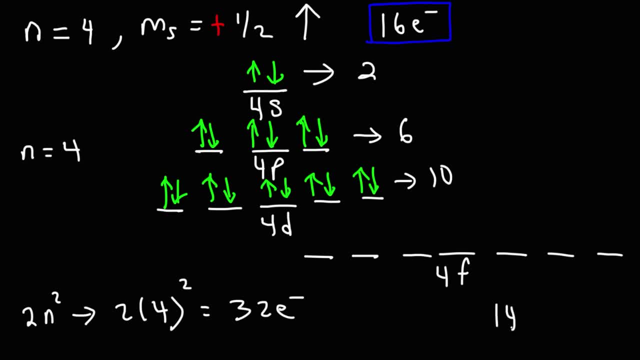 and then, if we fill this up, that's going to be 14.. 2 plus 6 plus 10, that's 18 plus 14, gives us 32.. And remember, half of the arrows will be up arrows. So half of 32 is 16.. 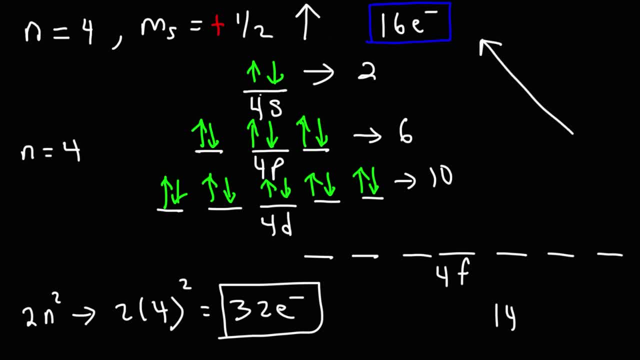 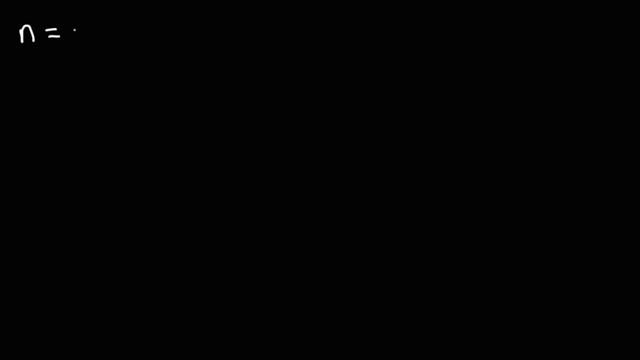 So that's the maximum number of electrons with these two quantum numbers can only be 16.. Now let's move on to the next problem. What is the maximum number of electrons that can have the quantum numbers n equals 4 and l equal 2?? 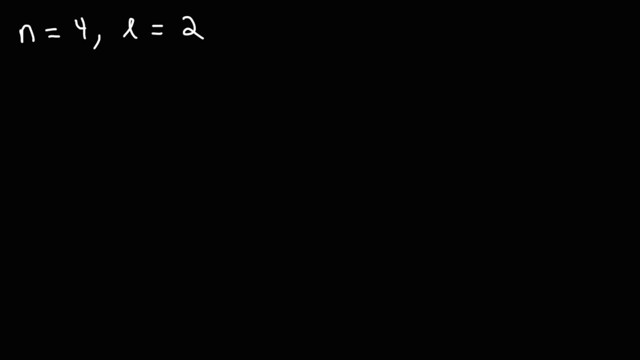 Now l, the angular momentum quantum number, tells you the shape of the orbital. When l is 0, we're dealing with an s orbital. When l is 1, we're dealing with a p orbital. When l is 2, it corresponds to a d orbital, And when l is 3, that corresponds to an f orbital. 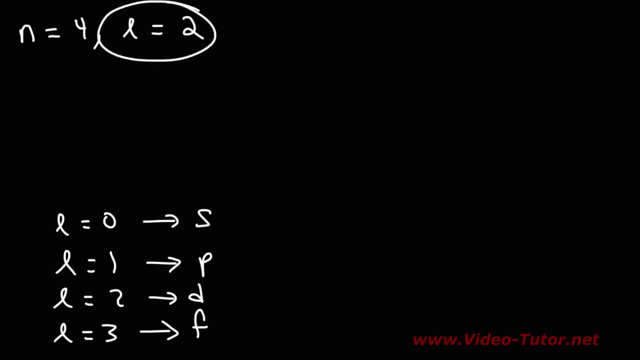 So here l is 2.. We're dealing with the d sublevel and it's in the 4th energy level. So that's, when you combine these two, we are dealing with the 4d sublevel. Now we know that s can hold up to 2 electrons, as mentioned before. 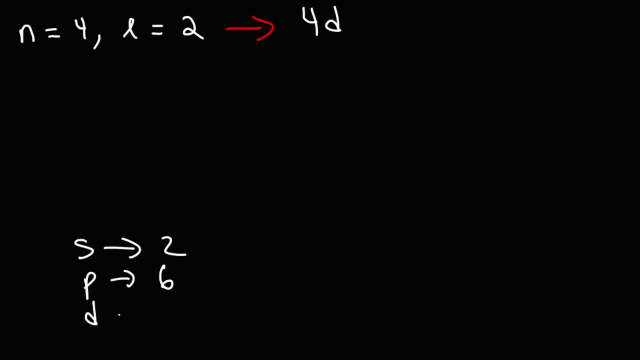 P can hold up to 2 electrons hold up a maximum of six electrons. d can hold up to 10, f can hold up to 14.. So the maximum number of electrons in the 4d sublevel is going to be 10.. Keep in mind, the d sublevel has five orbitals. 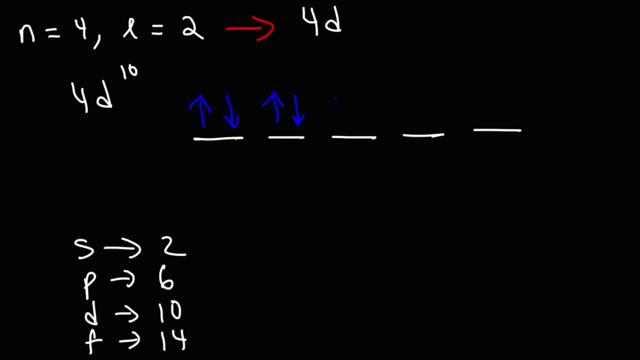 and each of these orbitals can hold up to 10 electrons. I mean each orbital holds up to two electrons, but five orbitals combined can give you a maximum of 10 electrons. So there's only 10 electrons that can have these two quantum numbers. So that's the answer for that problem. 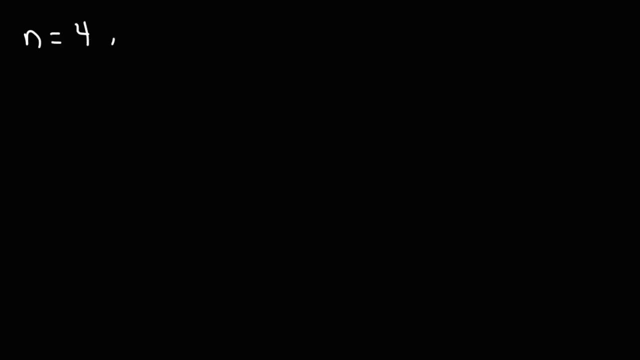 Now what if we have n and ml, the magnetic quantum number? What is the maximum number of electrons that can have those two quantum numbers In the fourth energy level? we know that there are four sublevels: s, p, d and f. Now the l value that corresponds to s, we said it's zero. For p, it's one, for d, it's two. 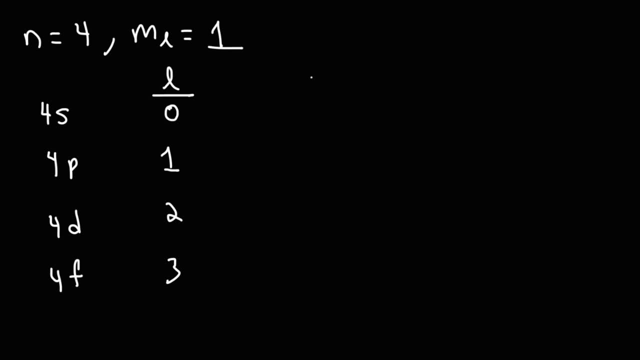 and for f, l is three. So that's the angular momentum quantum number. Now let's move on to the magnetic quantum number. ml is between a negative l and l. So when l is zero, ml can only be zero. When l is one, ml can only be zero. So when l is zero, ml can only be zero When l is one. 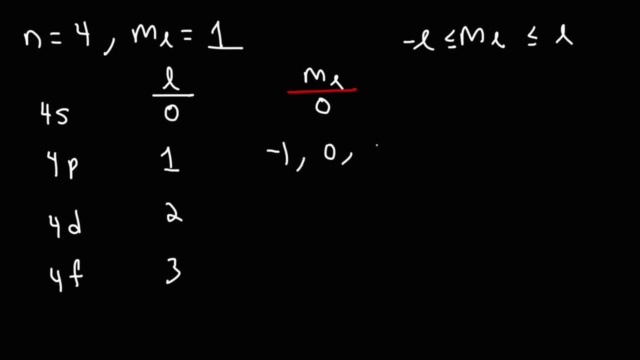 ml will vary between negative one and one. So it could be three things: When l is two, ml can vary between negative two and two, And when ml is three, it can vary between negative three and three. So we want to determine how many electrons can have an n value of four and an ml value of one. 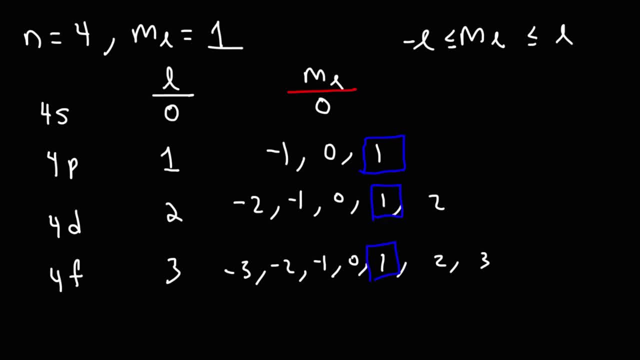 Here the ml value is one. Now recall that s corresponds to one orbital. p can have three orbitals, or rather it has three orbitals. d has five orbitals. Notice that ml corresponds to the orbitals in each sublevel, And we know that each orbital can hold up to three electrons. 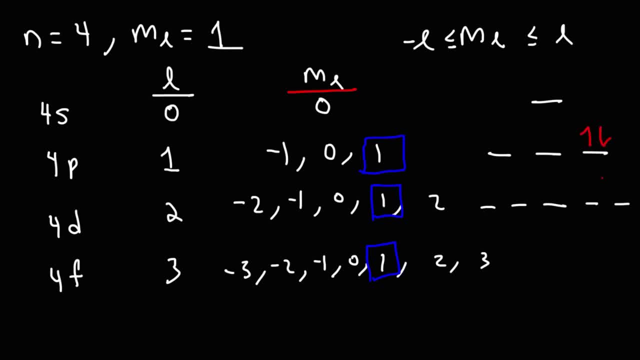 So this represents one orbital, And we know that each orbital can hold up to three electrons. This represents one orbital which holds up to two electrons. This represents another orbital which holds two electrons, And this represents one orbital in the f sublevel which holds two. 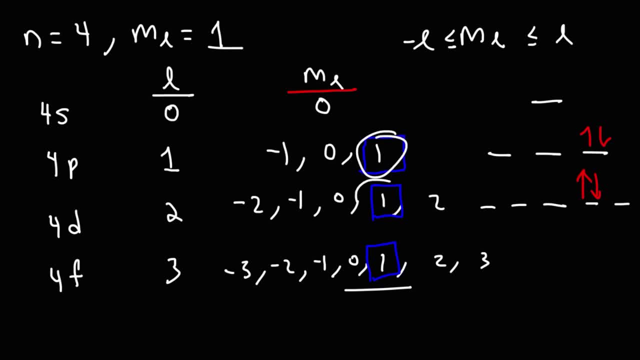 electrons. So because we have three orbitals circled, that corresponds to a total of six electrons. So that's the answer for this problem. That is the maximum number of electrons that can have these two quantum numbers. So far we've considered examples where we had two quantum numbers. But what if we have three? 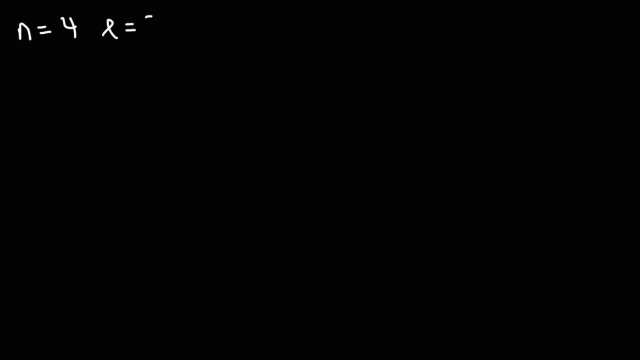 quantum numbers. Let's say n is four, l is three and ml, the magnetic quantum number. let's say that's a negative one. What is the maximum number of electrons with these three quantum numbers? Well, we know that when l is three it corresponds to the f sublevel. 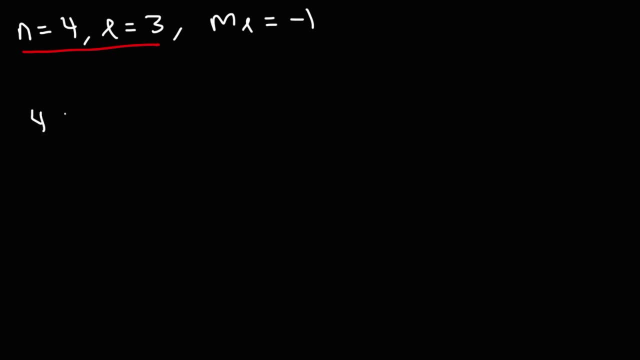 So the fact that n is four and l is three, we're dealing with the four f sublevel. f has seven orbitals And we know that when l is three, ml will vary between negative three and three. So each orbital has a specific magnetic quantum number. It has a specific ml value. 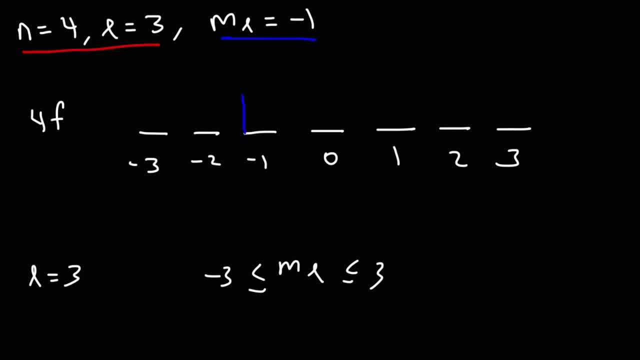 Now, ml is negative one, So we're focused on the negative one, So we're focused on the negative one. So that's why we've considered this problem. We've designed pointed Romeoked acytobe g, ue, r, T, f. 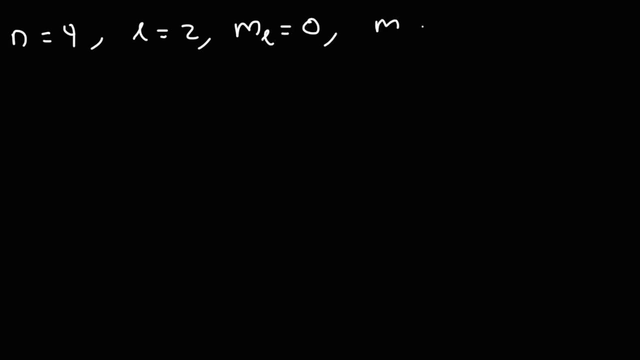 r, four quantum numbers? the answer is one, it's always going to be one. a set of four quantum numbers can only specify one electron each electron has. they all have their unique set of four quantum numbers. so anytime we're given four quantum numbers, if those quantum numbers are allowed, it can only represent one electron. 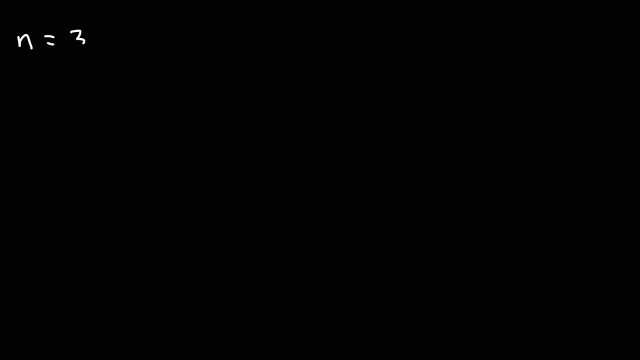 so let's go back to three quantum numbers. let's say, if n is three, l is one and the electron spin is plus one half, how many electrons can have these three quantum numbers? when n is three and l is one, what type of sub level do we have? 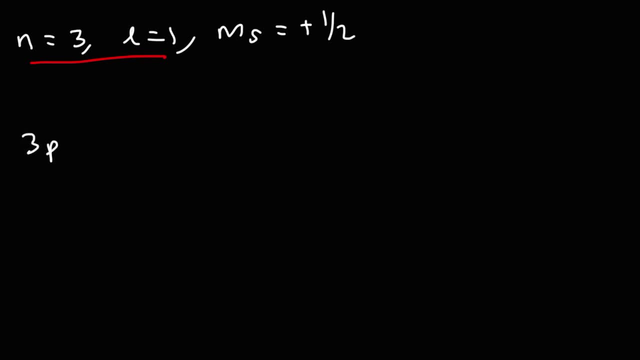 when l is one, it's the p sub level. so we're dealing with the 3p sub level, and p has many water levels. put theů three orbitals, So there's six electrons at most in the 3p sublevel. Now how many? 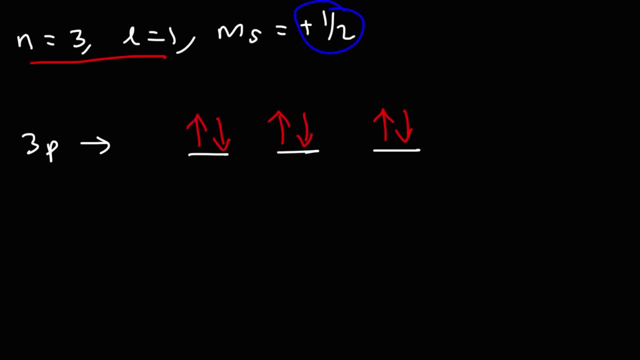 of them have a spin of positive 1 half. Well, these are only the up arrows. So there's only three electrons that contain these three quantum numbers. Now let's work on one more example. Let's say that N is 4,, ML is 1, and the electron 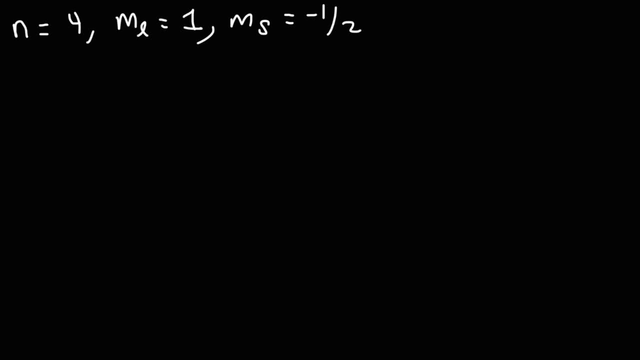 spin is negative 1, half. What is the maximum number of electrons that have these three quantum numbers? Well, we know that when N is 4, there's going to be four sublevels: 4s, 4p, 4d and 4f. And then we know that L is always 0,. 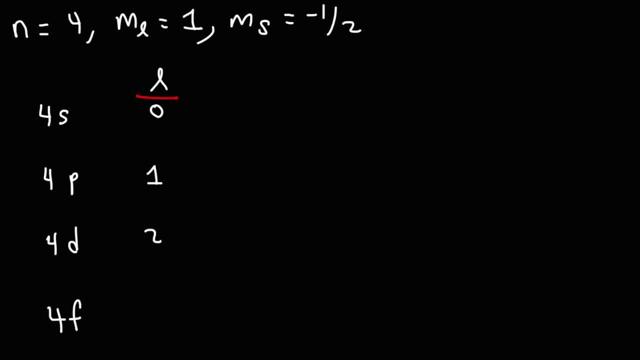 for S, It's 1 for p, 2 for d, 3 for f. Now let's focus on the ML values. S has only one orbital, p has three orbitals, d has five orbitals and f has seven. 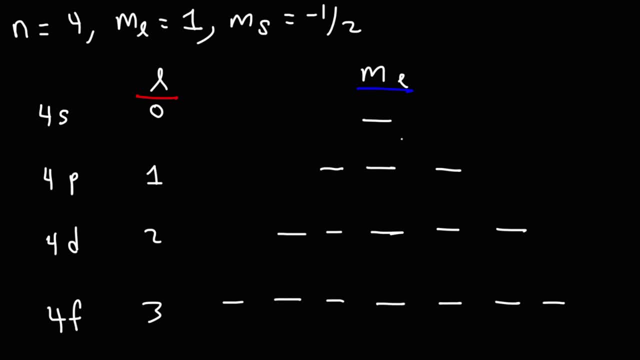 orbitals. Now, when L is 0, ML is going to be 0.. When L is 1, ML will vary between negative 1 and 1.. When L is 2, ML will vary between negative 2 and 2.. And you get the picture. So let's just put these: 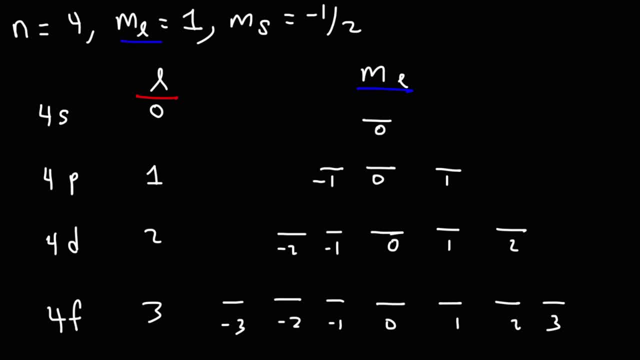 numbers in. And now we're focused on the orbitals with an ML value of 1.. So let's draw a box around each of those. Each of these three orbitals can hold two electrons, So this tells us that the There are six electrons with those two quantum numbers. 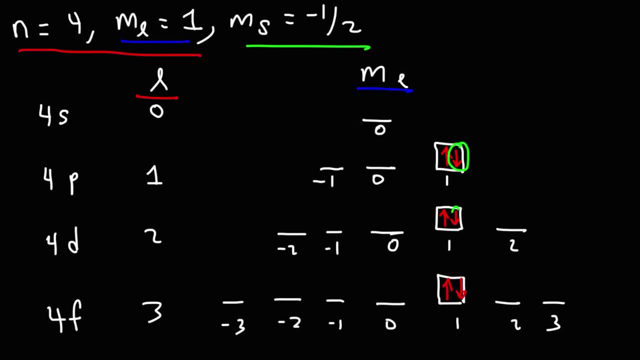 Now the spin is negative a half, so we can only highlight the arrows that are going down. So thus there's a total of three electrons with those three quantum numbers. So now you know how to determine the maximum number of electrons given a certain set of. quantum numbers. Thanks for watching.